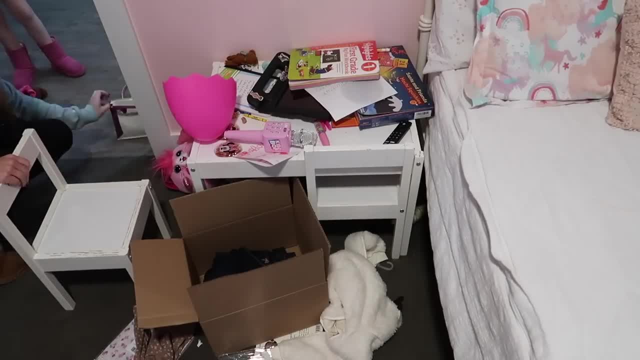 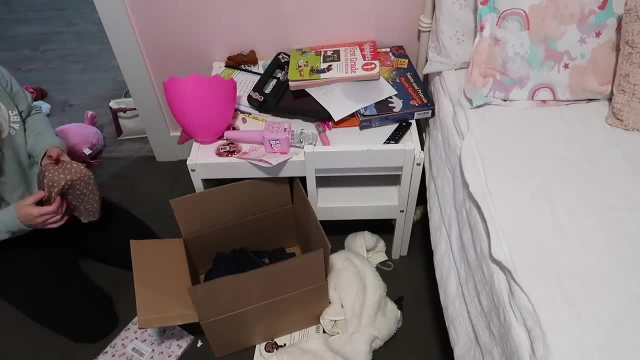 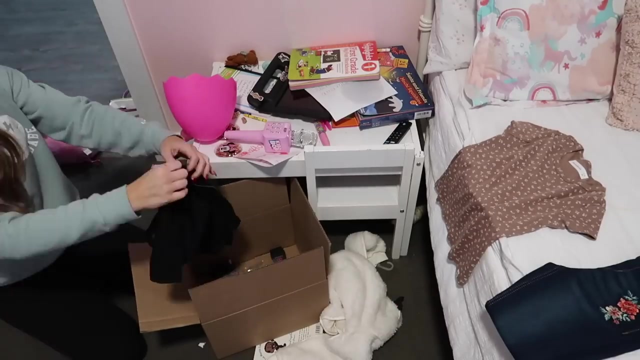 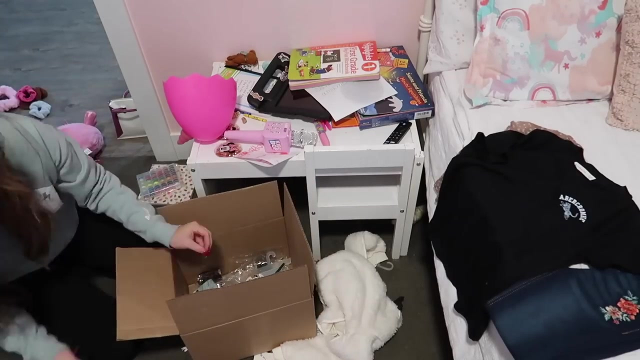 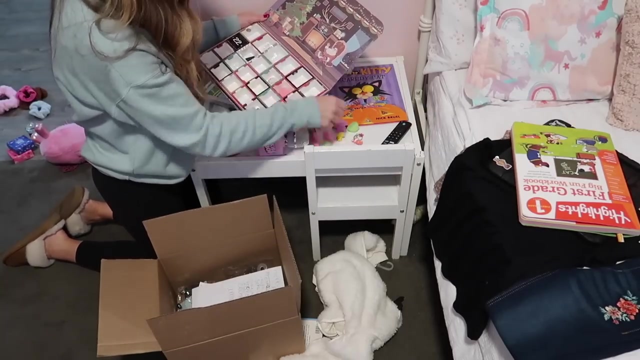 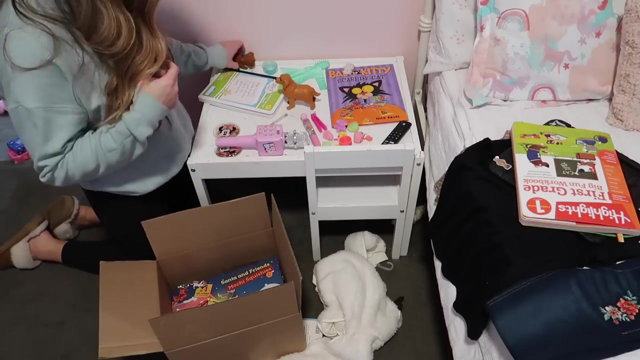 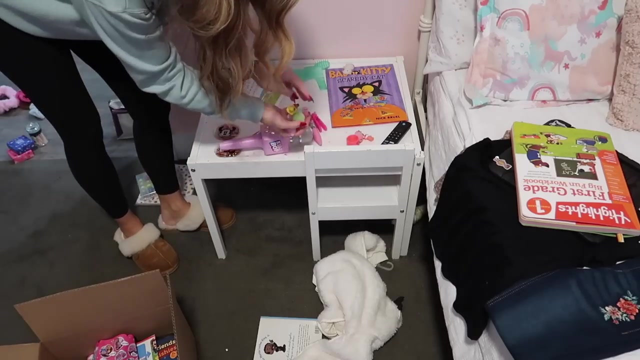 For you, for you, for you. I'm not gonna change. For you, for you, for you. I'm not gonna change For you. You might think I'm a little strange, but I'm not gonna change. You're drained by insecurities, While I see possibilities. You might think I'm a little strange, but I'm not gonna change. 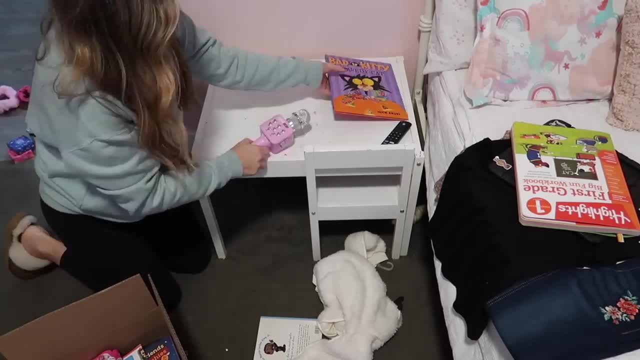 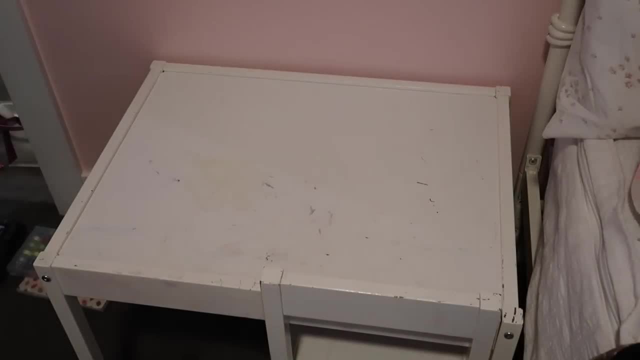 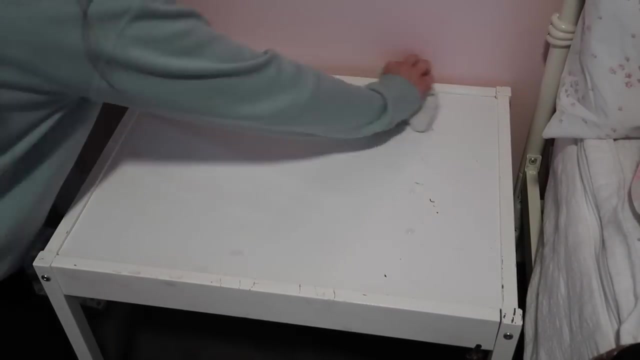 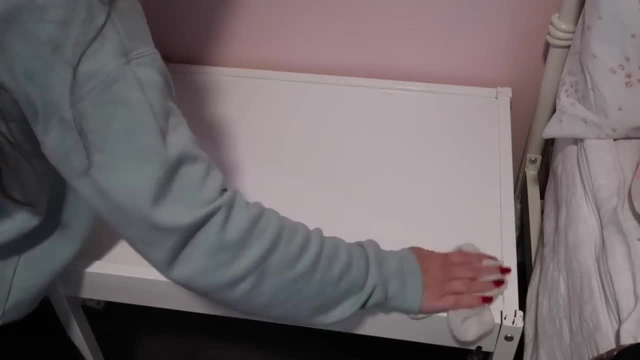 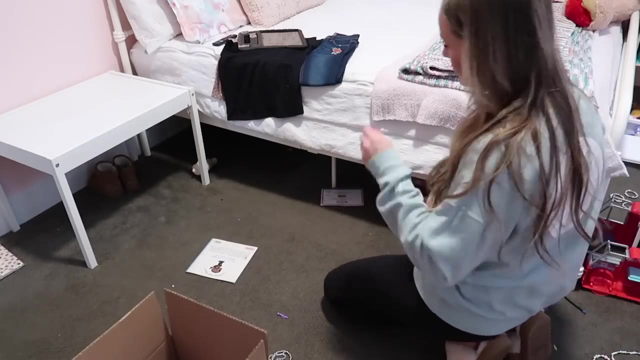 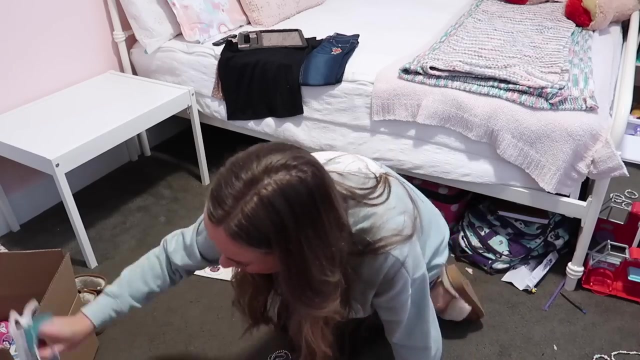 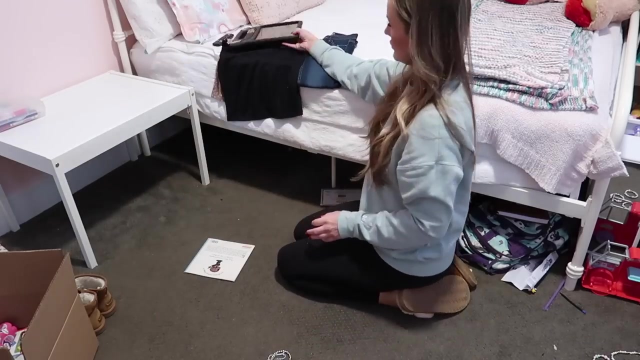 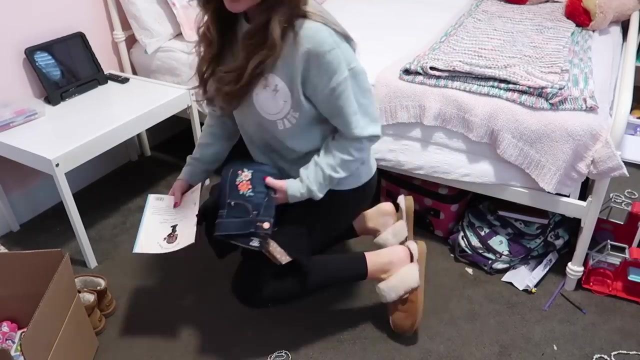 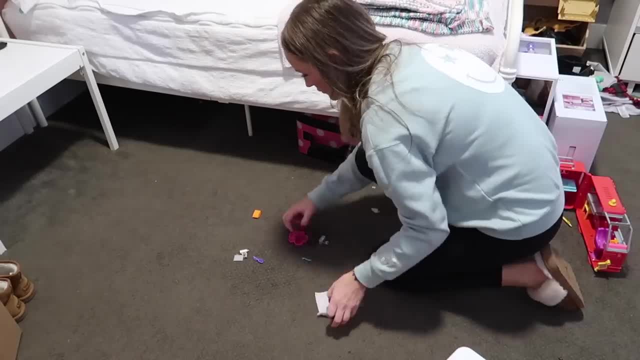 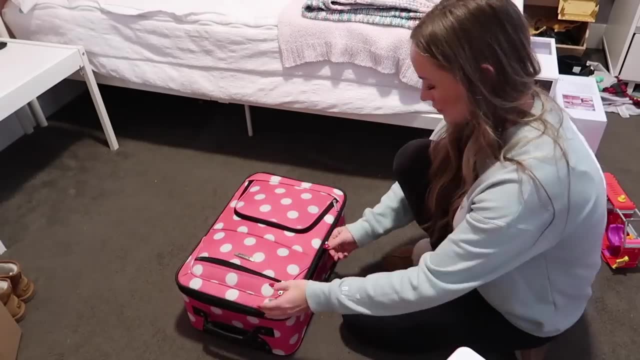 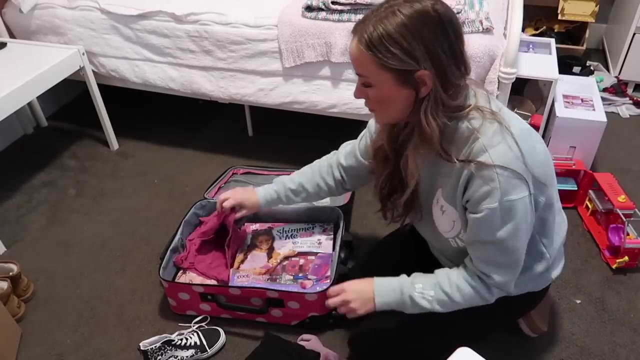 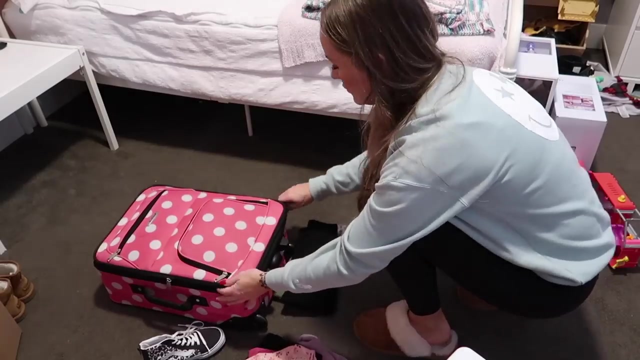 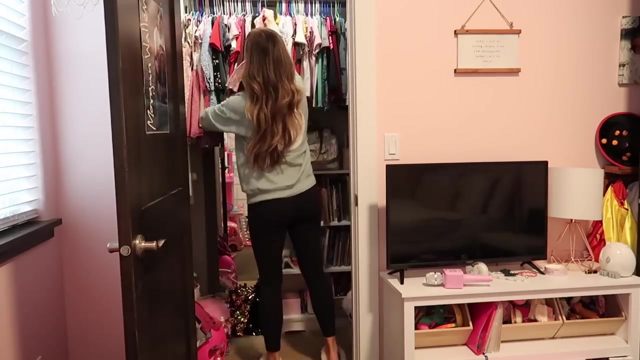 For you In our dreams. we always fight. We never worked it out. it just kind of slipped through our hands And I never really said that you hurt me. no one said. I just tried to understand. It was so exhausting so I lost it, had to make it stop. 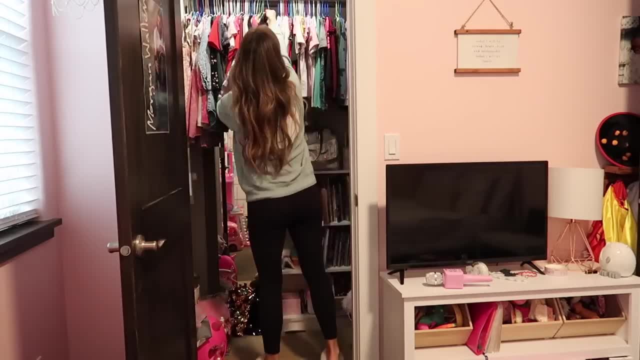 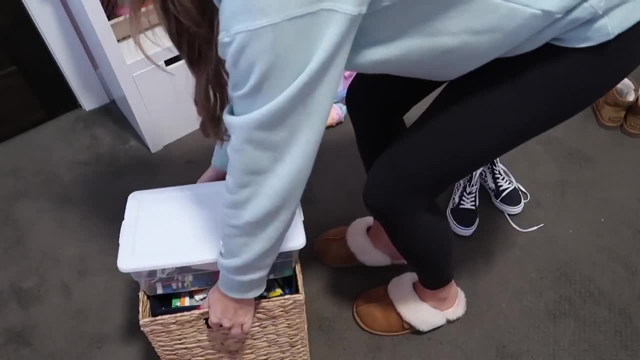 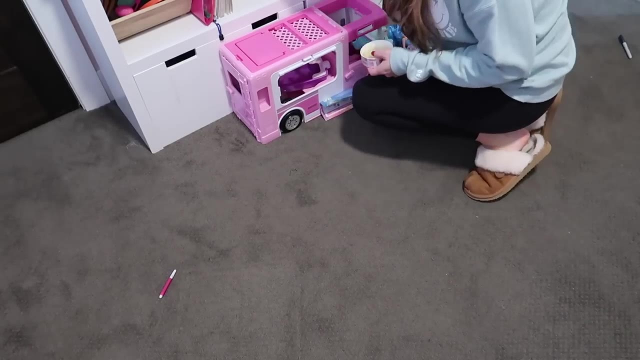 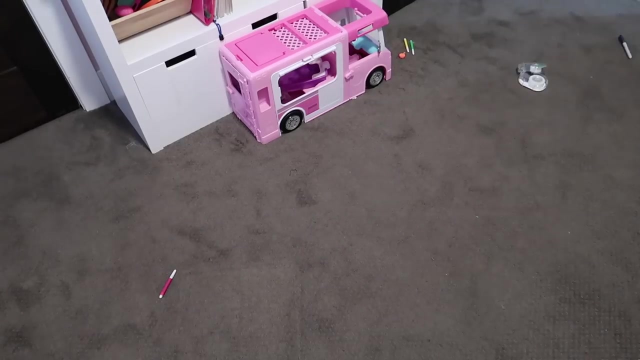 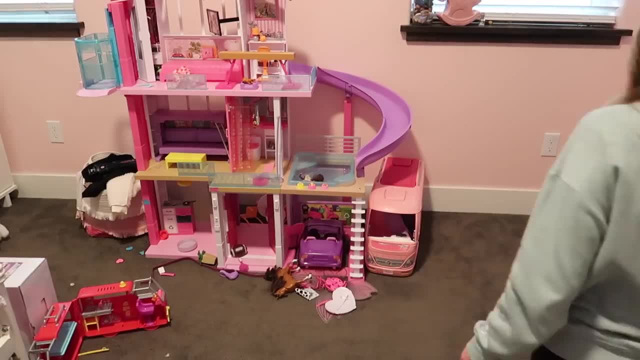 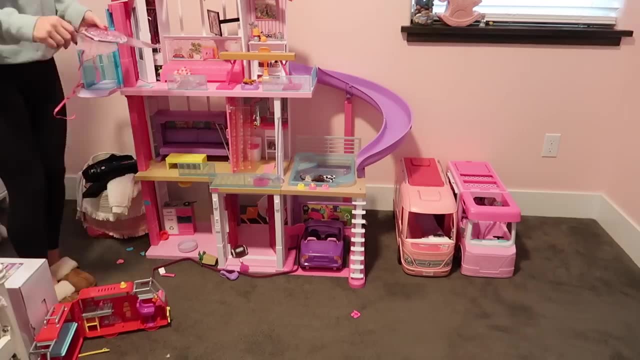 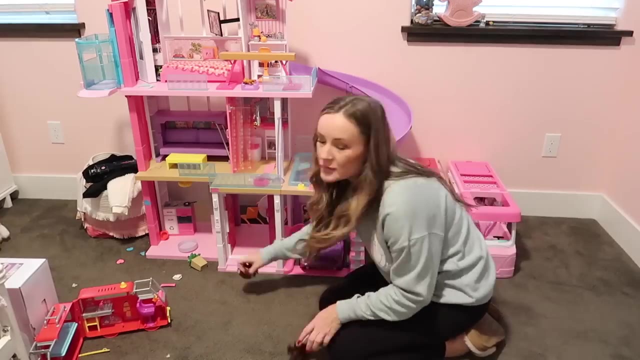 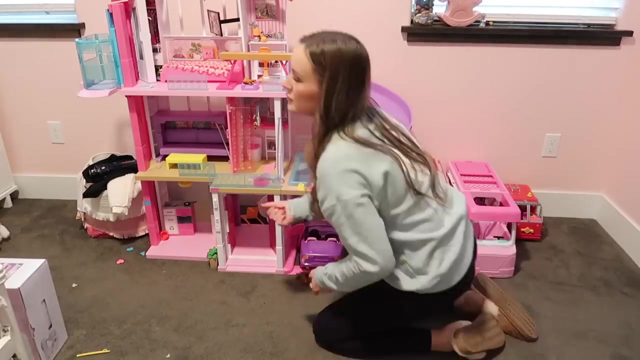 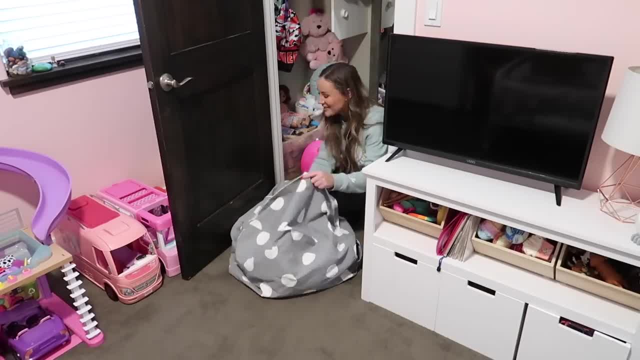 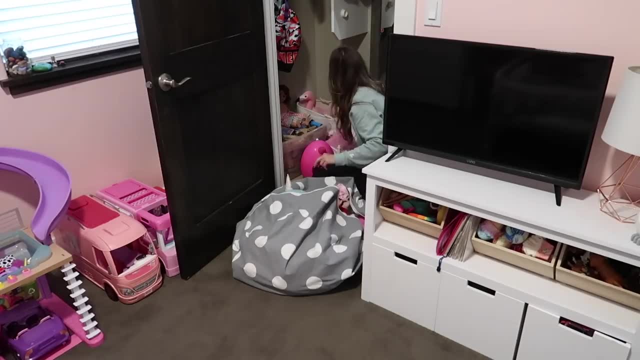 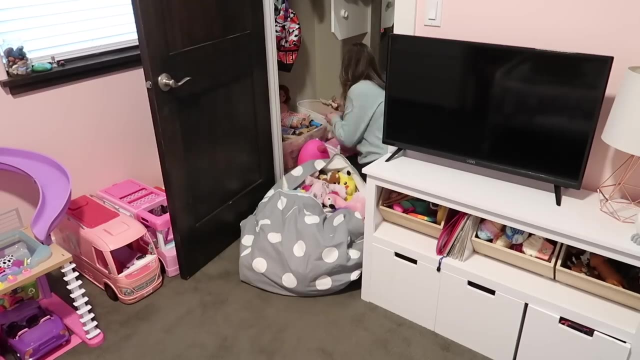 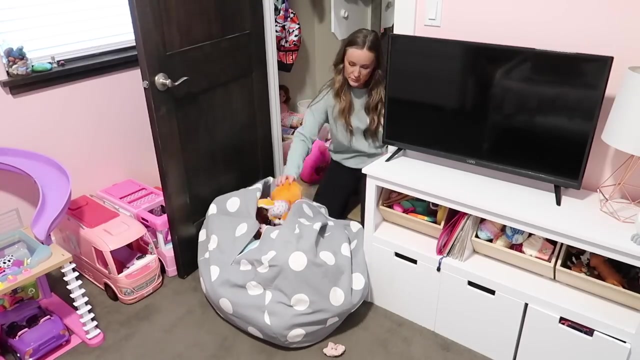 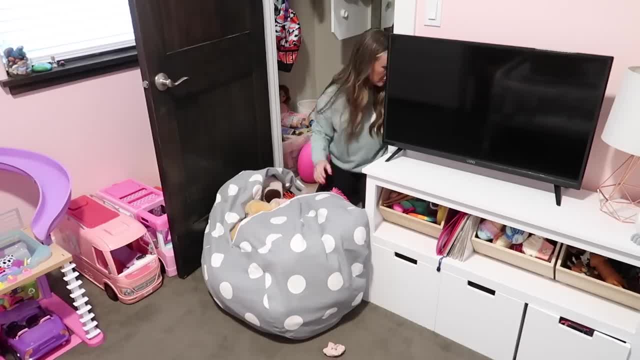 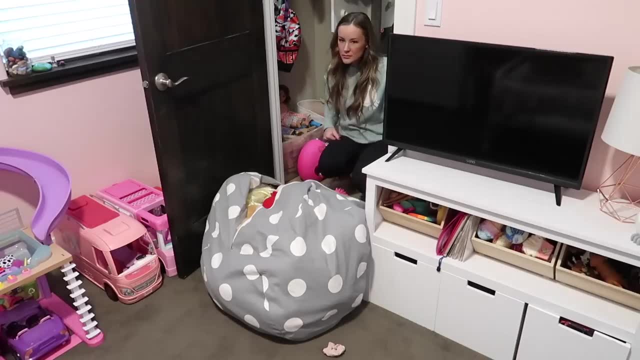 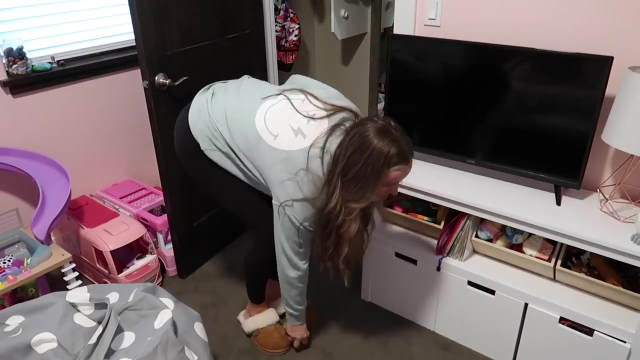 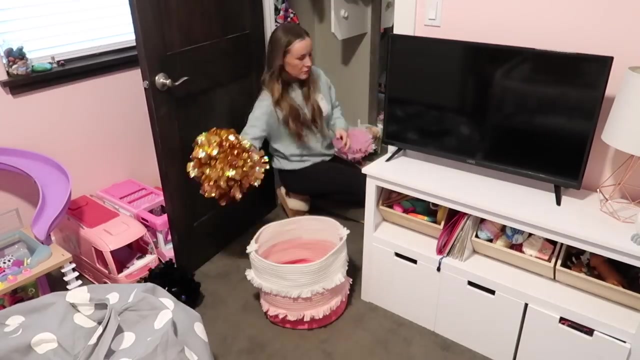 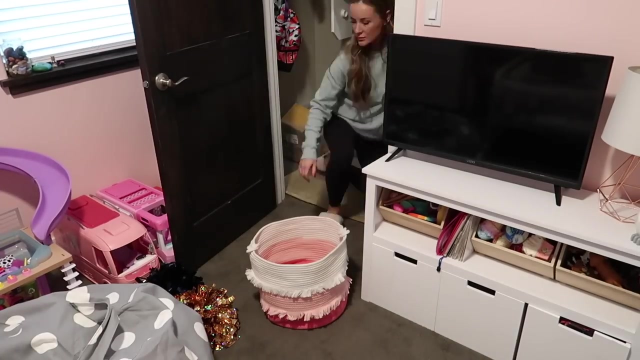 How it goes. Looking back, what a messed up time it was Figured out how to leave, and I'm glad because now I know. Oh, And when it was Such a bad plan Cause I really think I don't understand, I don't think It might really Push me away. 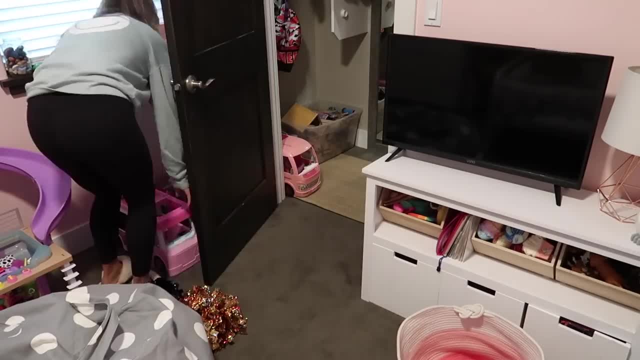 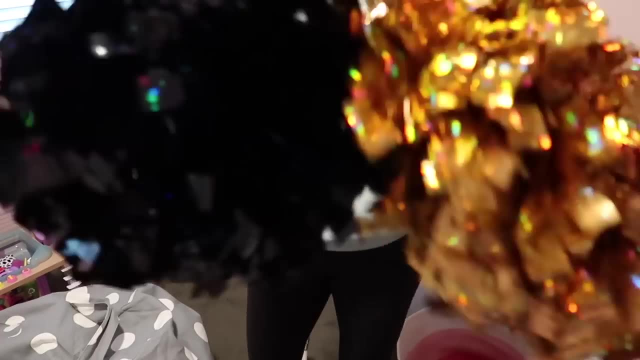 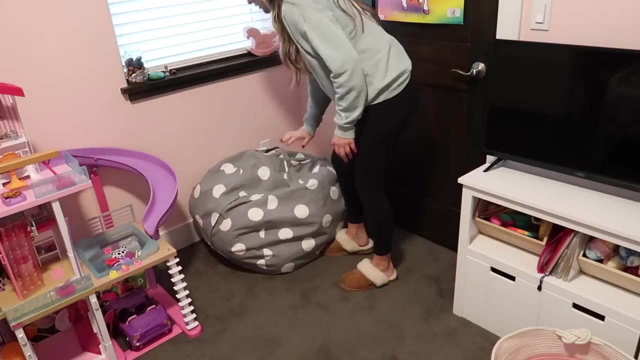 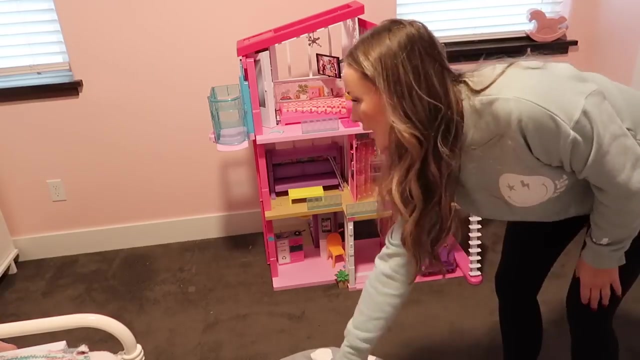 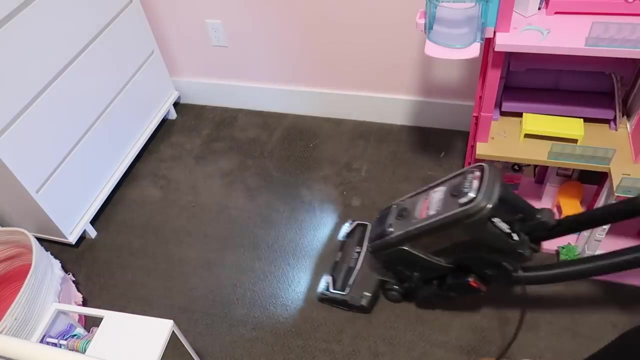 Away, Sleep When things run dry. I'm empty, I can't see. I'm blinded By this concrete And I should call you. See what you've been up to. I've been wondering: How far did you go In seven months? I bet you're happy And don't think that much about me. 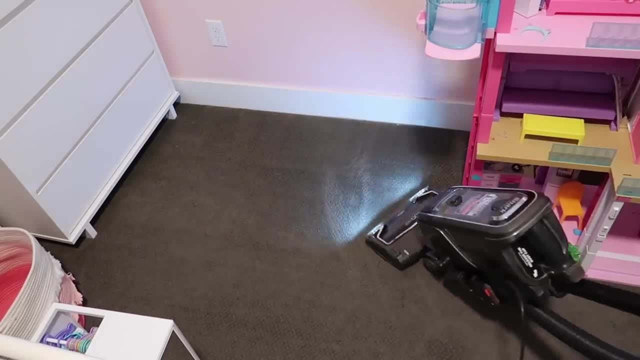 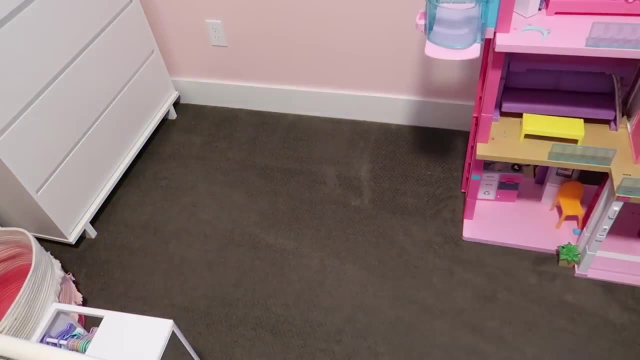 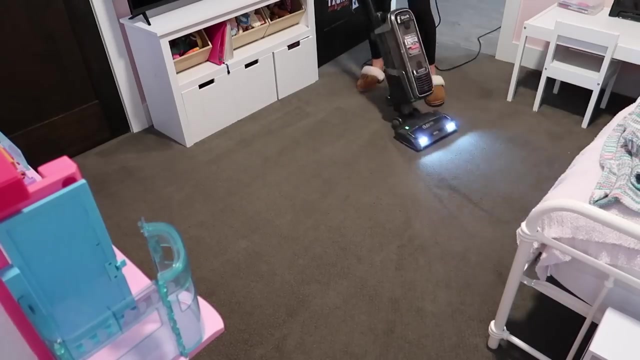 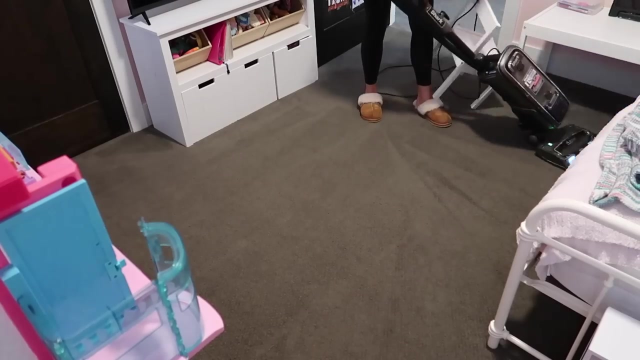 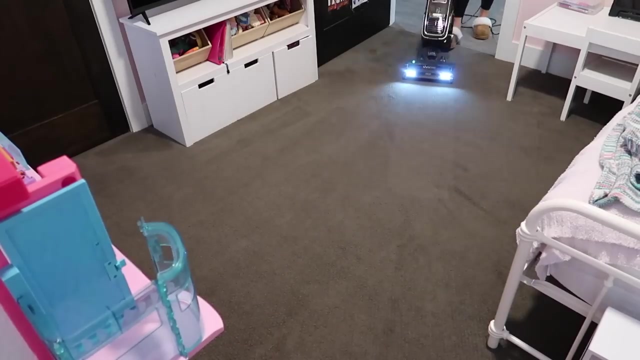 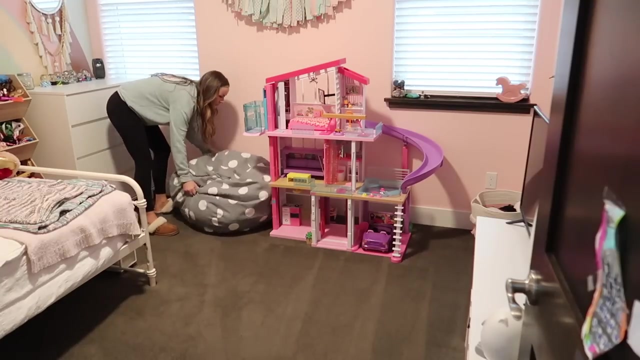 Here, I am not alone. I don't know No one Without you, You, You Without you, You, You, You, You Face Same old good Anxiety. Where's your irony? You Just smile Why? Cause I got everything I need, But not what I wanted. Alright, We are finished. My battery is about to die. 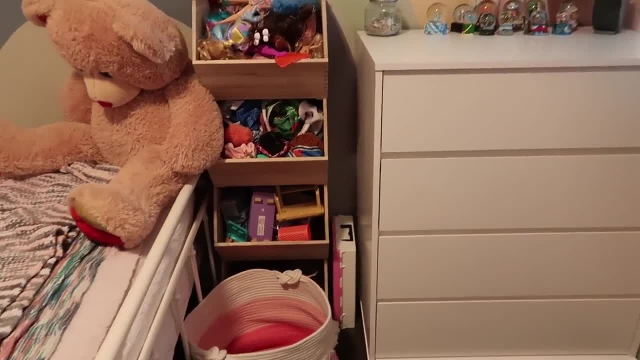 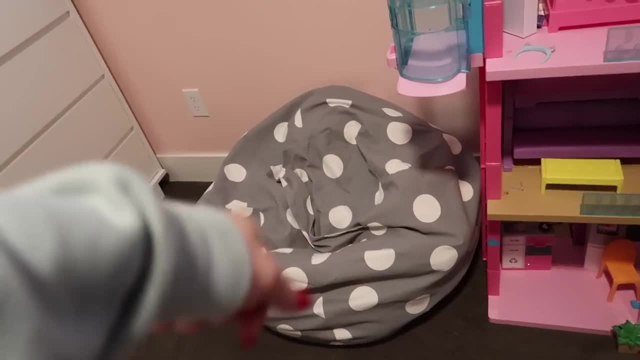 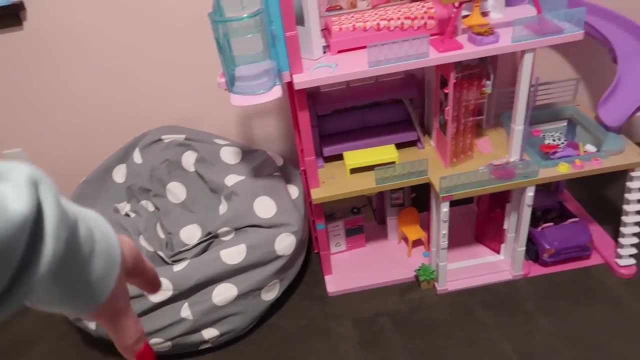 Made the bed And we have an empty toy box now Because all of these stuffed animals Are in this really cool bean bag Thing that I got For stuffed animal storage. She got that for Christmas, So we got all of our stuffed animals in there So she can sit on that. 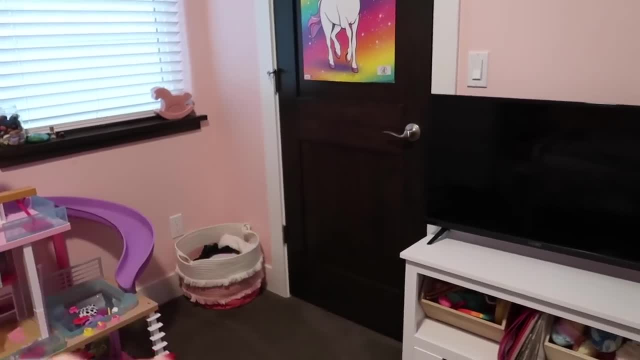 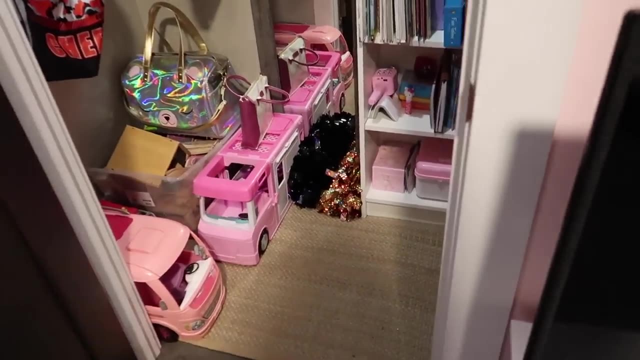 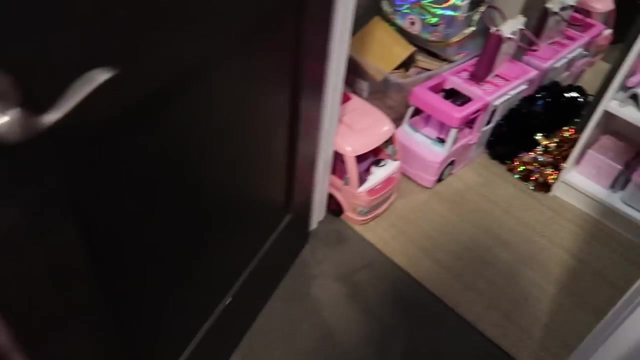 And see what she wants to eat, See her TV. We moved it Because it was too big to go in this corner. Dirty clothes basket over here And then her closet was already clean. I just cleaned it the other day. I just kind of reorganized Because I took all the stuffed animals out. 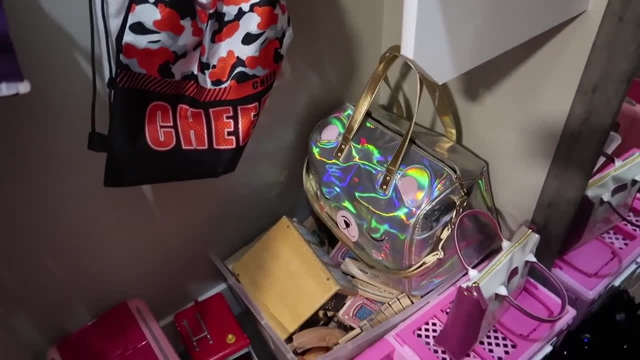 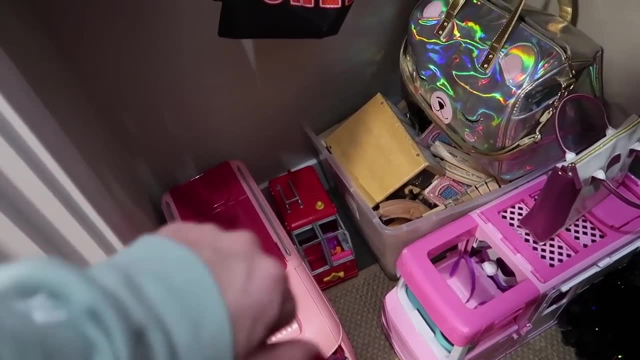 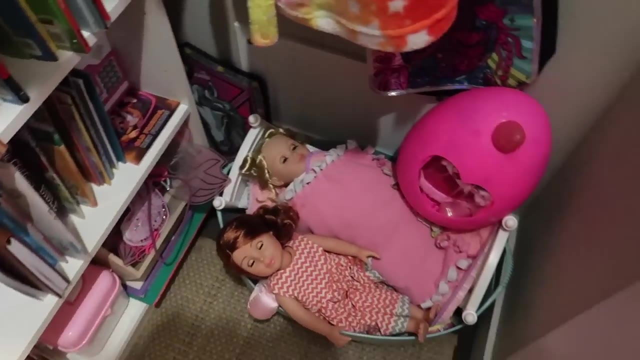 So we got her train tracks, Her cheer bags, Both of her RV camper Or her Barbie Barbie RVs, And then her Barbie fire truck, Her palm. This is all her. My battery did in fact die. Anyways, Dolls here, Books and toys. My mom got her a sewing machine. 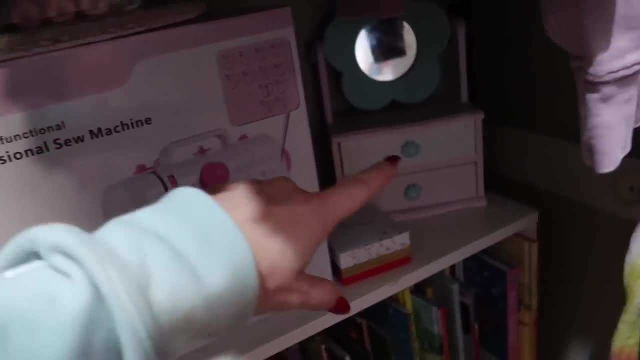 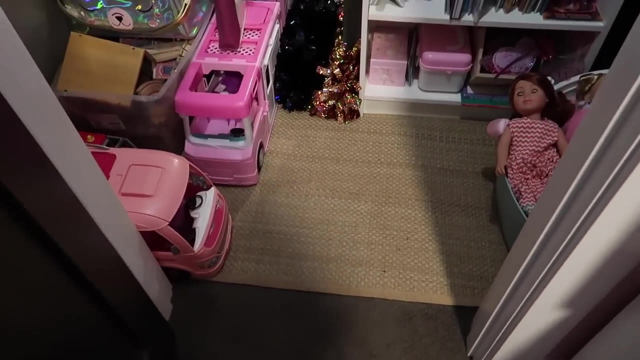 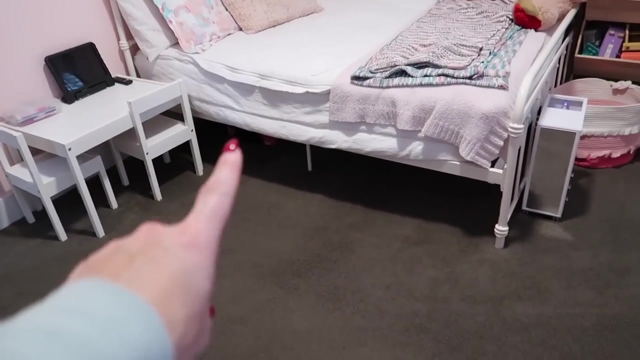 For Christmas. We have her sewing machine stuff up here- Jewelry box, Her mirror, Clothes- And then she also gets in there and reads her books And stuff. Floor is all clean, Under the bed is clean. you just keep her suitcase under there And her tumbling mat Washed off the 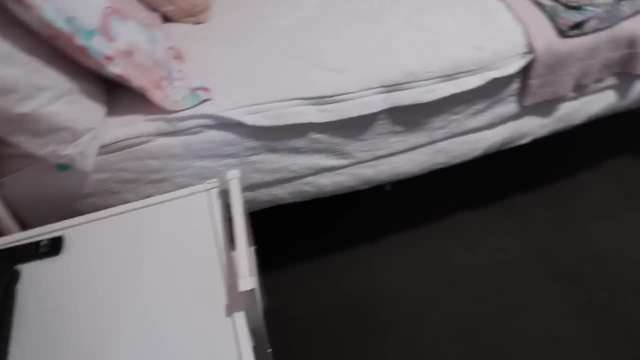 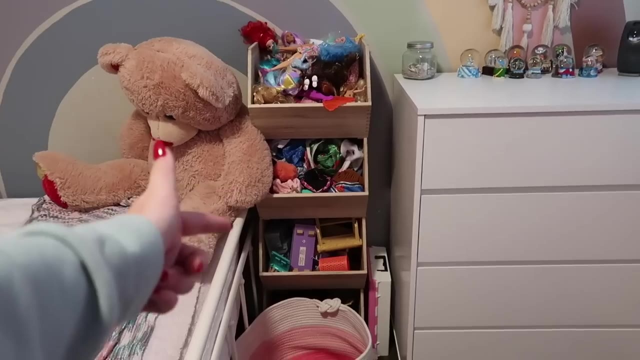 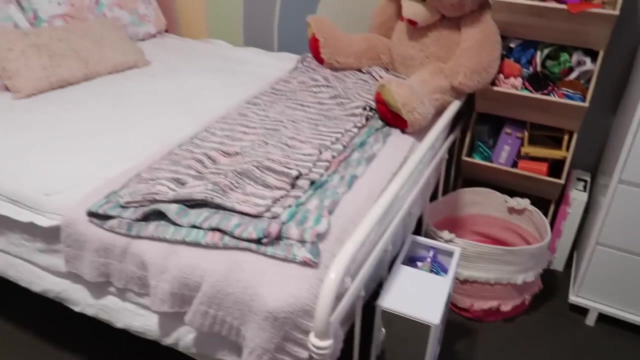 Or wiped off the table, Got that all clean And all of this stuff was already organized: Barbie's doll clothes, Barbie furniture And spirit horses down there And then just Some doll clothes storage. So Her room is clean. She has her door decorated, But anyways we got to get ready to.